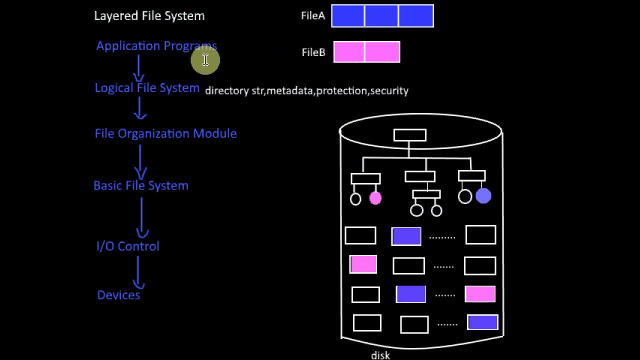 the symbolic name, which is obtained from the upper layer. the file will be located in the directory structure and the metadata is accessed. The information regarding the file, such as size of the file or the file size, is also available. The file is then stored in the. 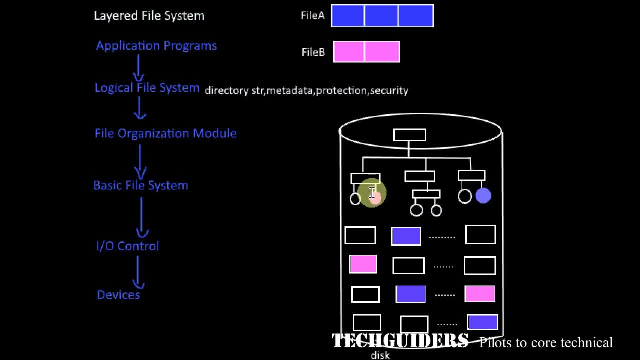 directory and the data ownership permissions and even the actual disk location etc. are accessed. Thus, if one user tries to execute something which is beyond his permission on the file, the access will be denied at this level itself. Hence this layer is also responsible. 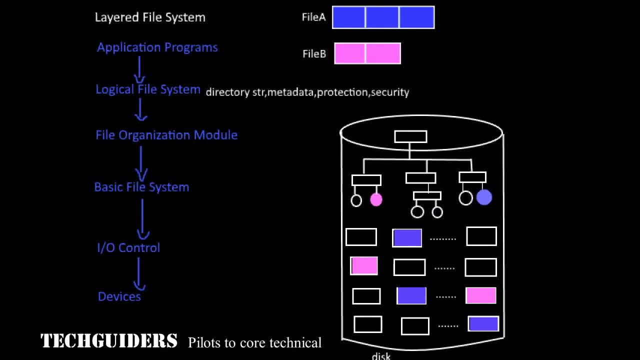 for protection and security. Next layer is file organization module. Now the information regarding the files, including the disk location of the file, is accessed from the upper layer. Using this information from the upper layer, the file organization module maps the logical address, the logical block address, into the corresponding physical 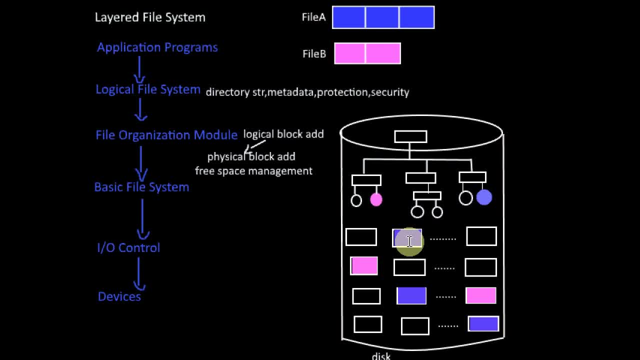 block address. It also performs the free space management by tracking the unallocated blocks and providing these blocks to the files as needed. Next level is basic file system. Now, by knowing the physical block address and the requested user operation from the upper layer. this layer issues generic commands to the underlying 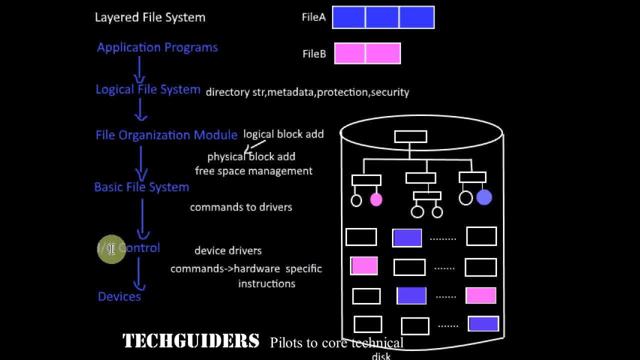 layer And the underlying layer is the IU control layer, which consists of the device drivers and interrupt handlers. It translates the commands from the upper layer to the hardware specific instructions which the IU devices can understand. Finally, the lowmost layer consists of the physical devices, which follows these hardware. 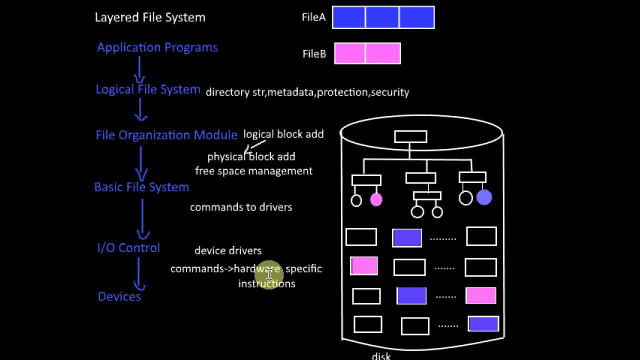 specific instructions and execute the required function. Next, let's look at the hardware.